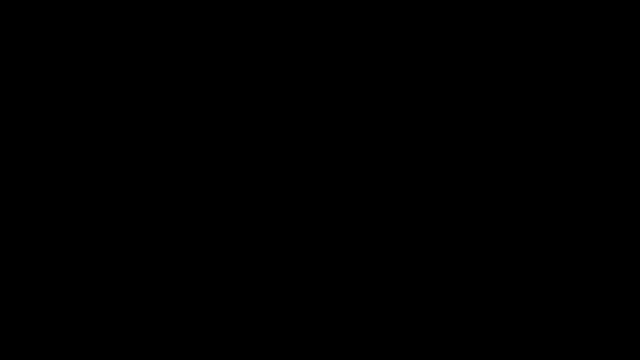 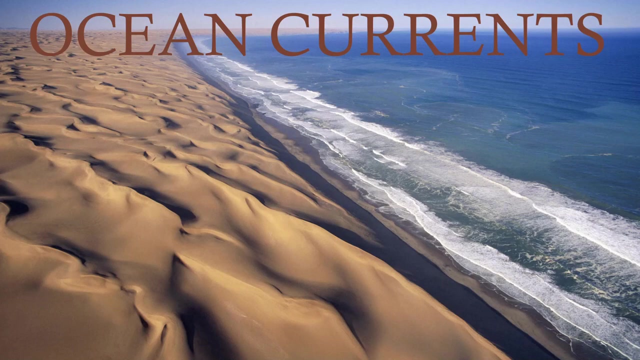 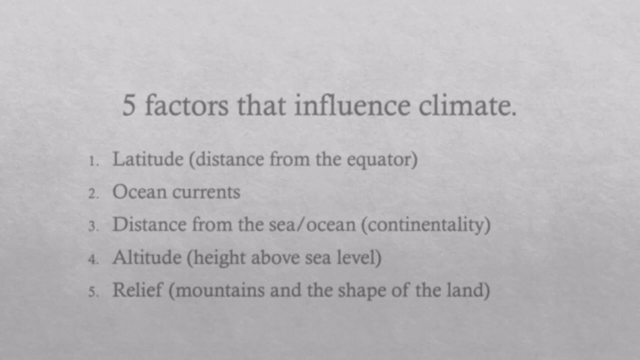 Hello and welcome. In this video, we are going to examine how ocean currents affect the climate of coastlines they flow past. Before we get into that, let's just remind ourselves about the definition of climate, as well as the factors that affect global climate. Climate is best. 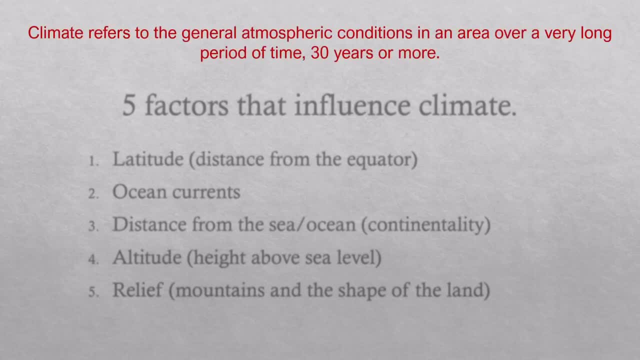 defined as the general atmospheric conditions over a place over a minimum of 30 years or more. The five factors that affect climate are: latitude or distance from the equator, ocean currents, which we are going to examine in this video, distance from the ocean or. 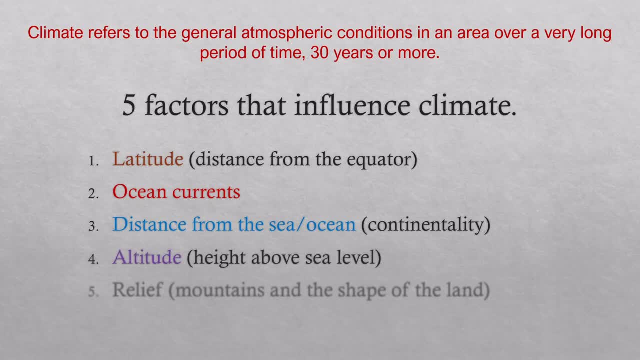 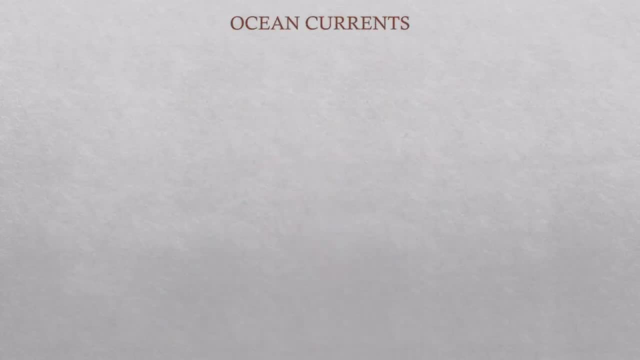 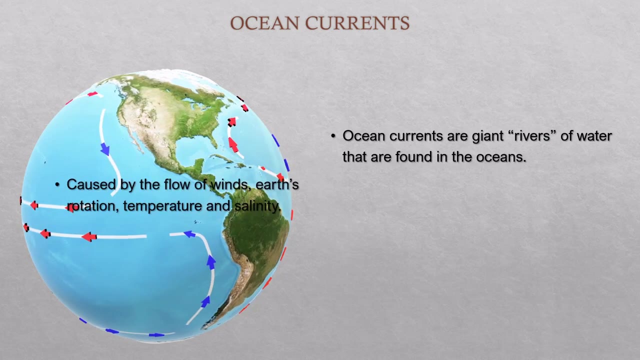 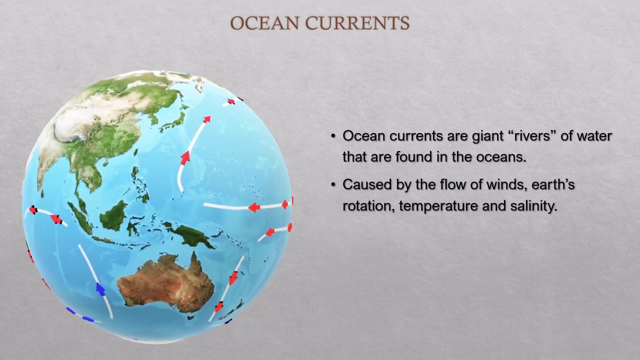 continentality, altitude, also known as height above sea level, and relief or the shape of the land. Ocean currents are giant underwater rivers or conveyor belts of water that flow in the oceans. There are many contributing factors that create these ocean currents. Some of these include the winds, earth's rotation, the temperature of the water. 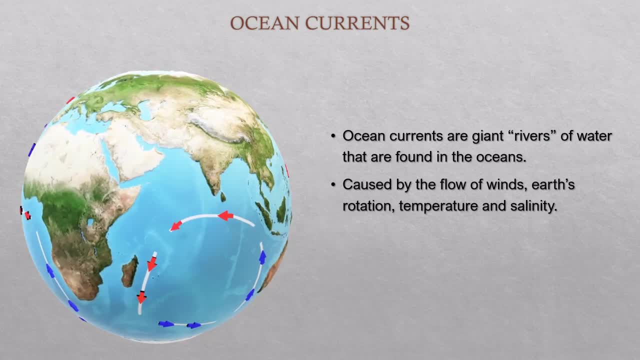 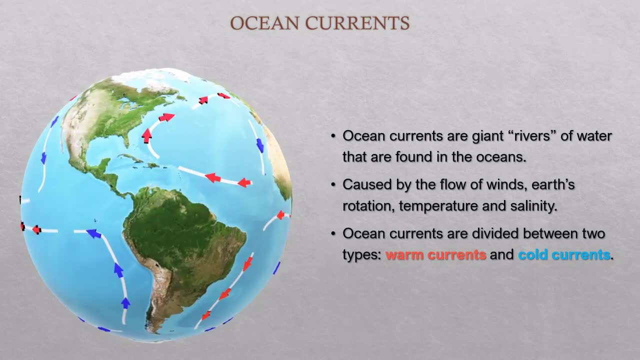 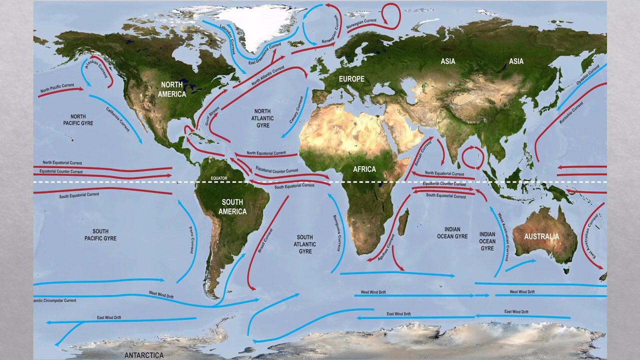 and the salinity or salt content of the water. There are two categories of ocean current – warm currents and cold currents. This map of the major global ocean currents shows something quite important that we should take note of. Warm ocean currents originate at the equator and transport warm water south and south. This intensity of the ocean currents is theọrichescotft n the edge of the ocean, and that's when we think about the associate forces of the ocean currents. 뜻 tema Kody et al is, though we are going to get inside and have a closer look as we go beyond the ocean limits. 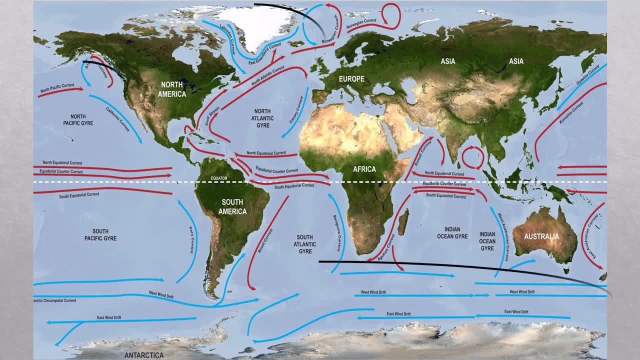 in the ocean. We are currently looking at the mothership, For example, we'd like to identify north to the high latitude, and cold ocean currents originate at the high latitudes and transport cold water towards the equator. From this map, you can also identify some global 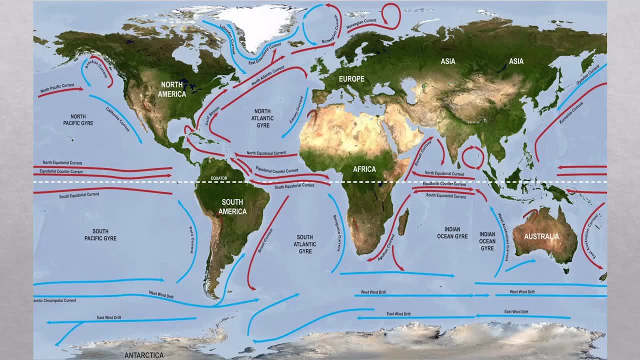 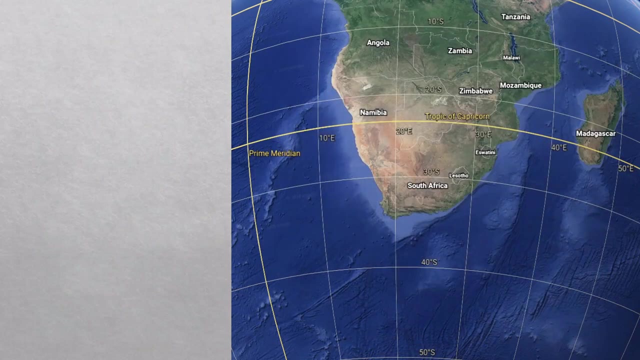 climate patterns created by ocean currents. Almost all coastlines where major cold currents flow are dominated by a light brown color that, on this map, indicates a lack of vegetation. These regions are deserts. Let's look at the effects of ocean currents by examining the 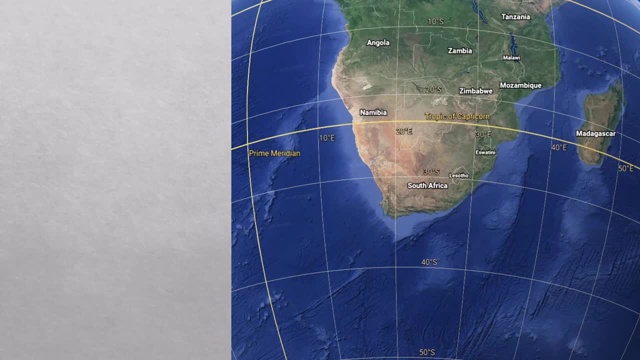 effect they create on the coastlines of countries or regions. A perfect example to use here is the southern African region. Situated to southern Africa's east coast is the Indian Ocean, and along the west coast you can find the South Atlantic Ocean. Both of these oceans have a massive impact. 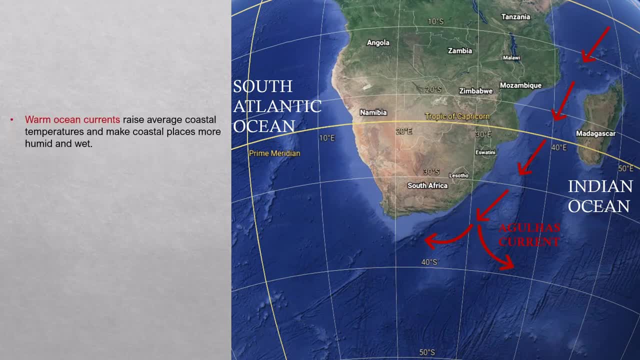 on the climate of southern Africa. The current flowing through the section of the Indian Ocean that borders southern Africa is the warm Agulhas current. This current moderates the east coast temperatures as it provides a constant flow of warm water from the equator, which leads to lots of evaporation. 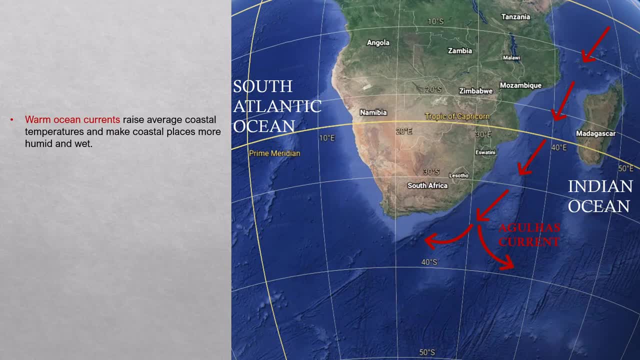 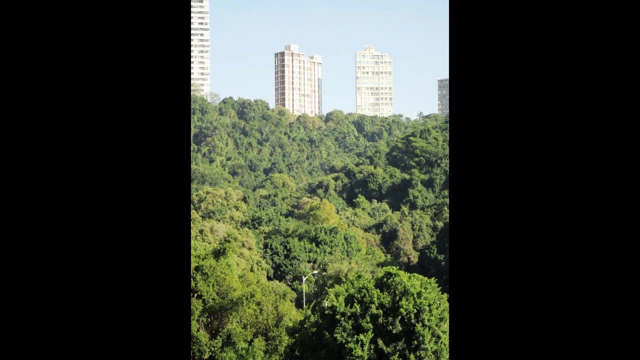 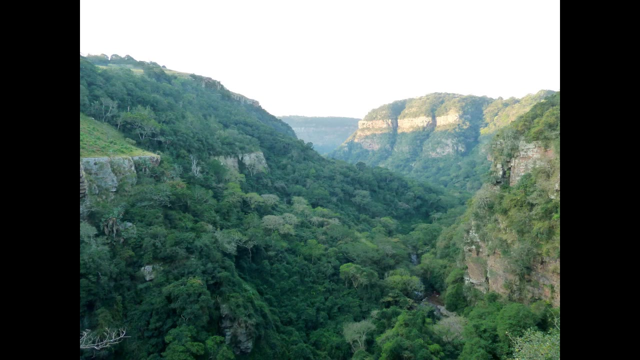 occurring off this current. As a result of this, places along the east coast like Durban have humid summers with lots of rainfall. As you can see from the pictures, southern Africa's east coast also has a lot of green vegetation. This picture shows the Kranskloof nature reserve and you can see the densely packed trees and greenery. 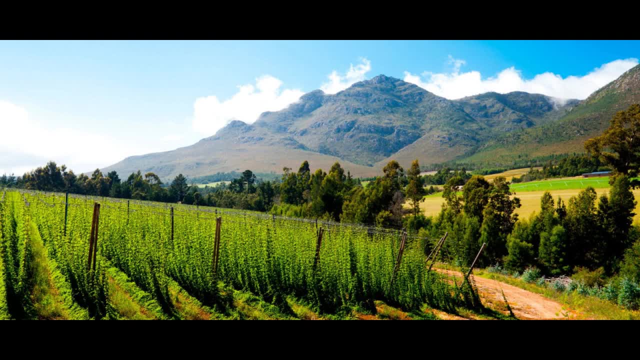 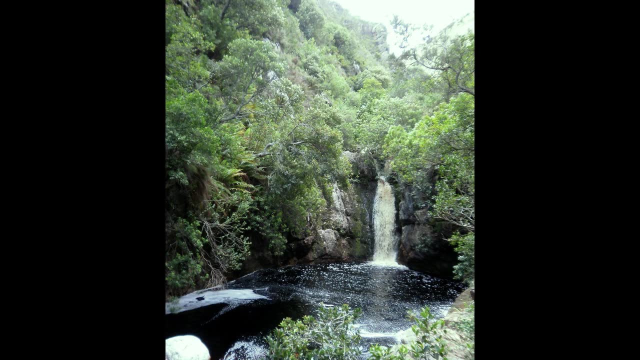 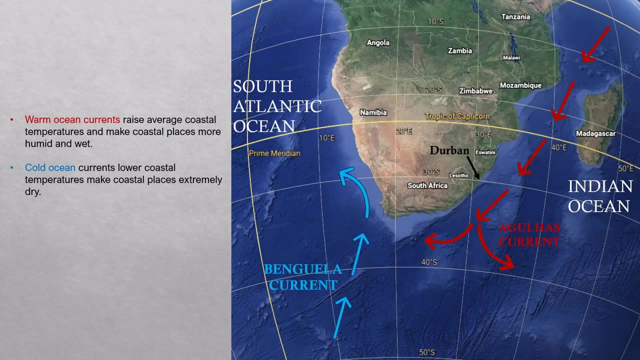 everywhere. George, which is another town along the east coast, is well known for its beautiful green scenery, which it can also attribute to the warm Agulhas current. The current flowing in the South Atlantic Ocean is the Cold Benguela current. This is 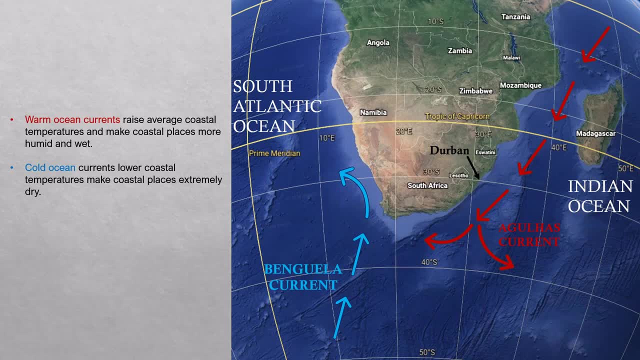 one of the coldest and the most wetest deserts in the world, and the current is often worse than the other two. The coldest days of the year are the coldest. The coldest days of the year are the coldest days of the year. It's usually about 1.5-2pm. 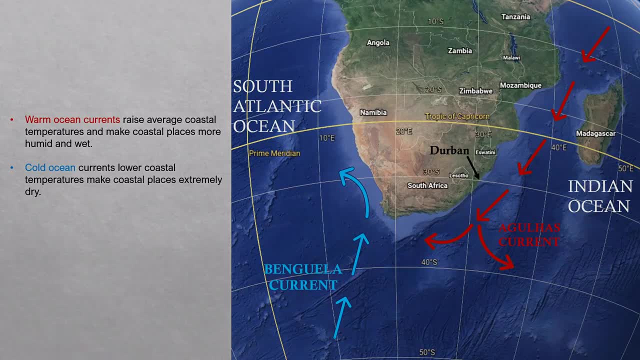 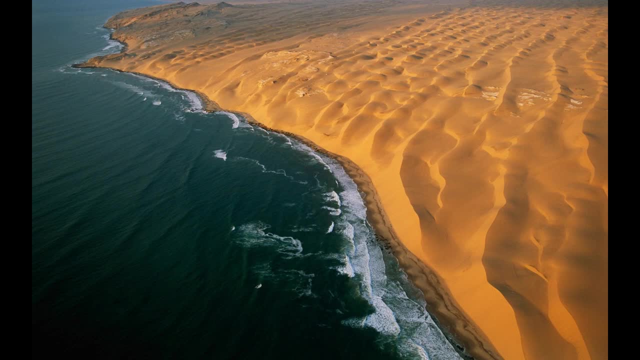 This current brings cold water from the south pole. Due to the cold temperatures of the water, very little evaporation occurs along this coastline and the climate is extremely dry throughout the entire year. The west coast of southern Africa is dominated by the Namib desert, which is widely thought. to be the oldest desert in the world. Estimates put its age at around 55 million years old. It is also one of the driest deserts in the world and the coldest in the entire Arctic. It is also one of the driest deserts in the world and it's known as a desert of climate change. 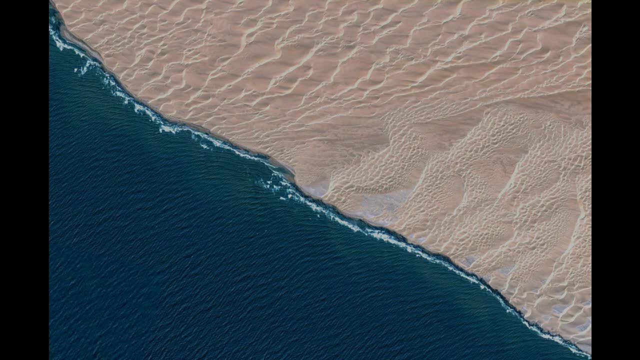 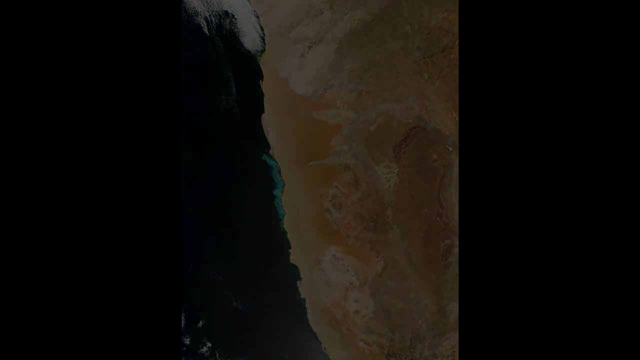 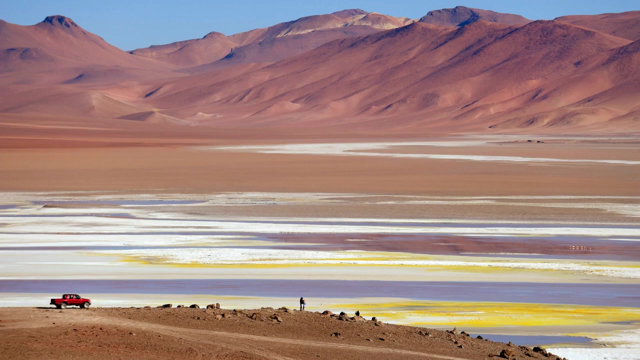 deserts in the world and very few people inhabit it. While the scenery of the Namib lacks the greenery and vegetation that doesn't make it any less magnificent to look at, The west coast of South America is also dominated by a desert called the Atacama Desert. The west coast of North America contains the 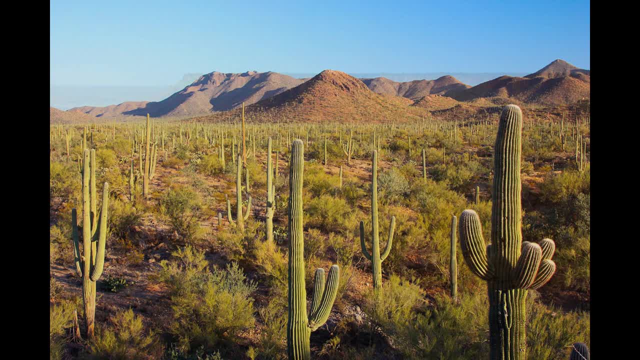 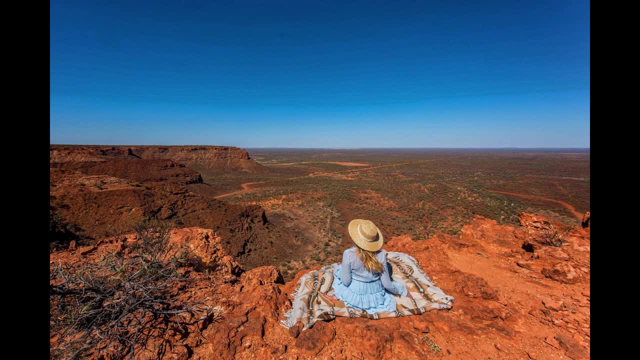 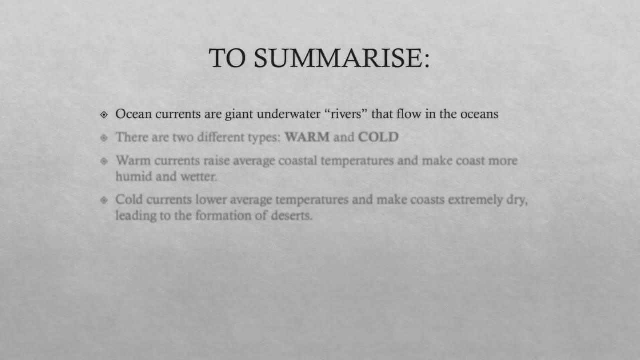 Sonoran Desert and the west coast of Australia sees the early parts of Australia's outback, which is a large series of interconnected deserts. Before we finish the video, let's just summarize what we have learned. Ocean currents are giant underwater rivers that flow in the oceans. There are two different types of